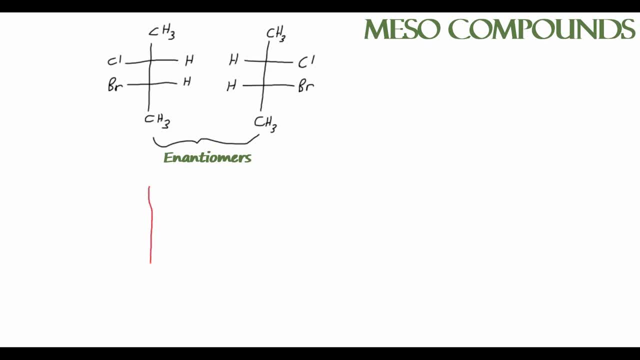 expect. However, what if we draw a the same sort of skeleton, except now we have two bromine substituents on the same side? Well, we can again draw the mirror image of that Fischer projection with the bromines on the other side of the molecule. but you can also notice that these two molecules are actually the same If you rotate the. 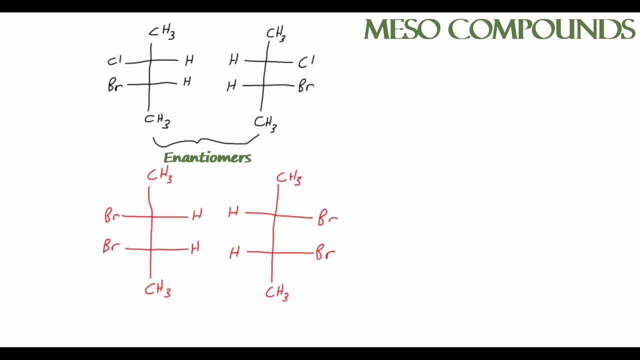 first one by 180 degrees, you'll end up with the second Fischer projection. And again, if you remember from Fischer projection, 180 degree rotations result in this same molecule. So what's interesting is that these molecules are actually the same one, even though they are mirror images, And that is because we have this plane of 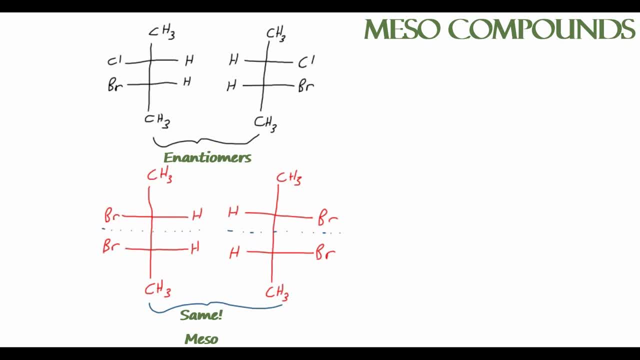 symmetry, Because the molecule is symmetrical. we have the same substituent on carbons two and three here. That is what we call a mesocompound. So it has two stereocenters, but it is symmetrical, which means that it does not have an enantiomer. So, as a definition, mesocompounds are compounds with more. 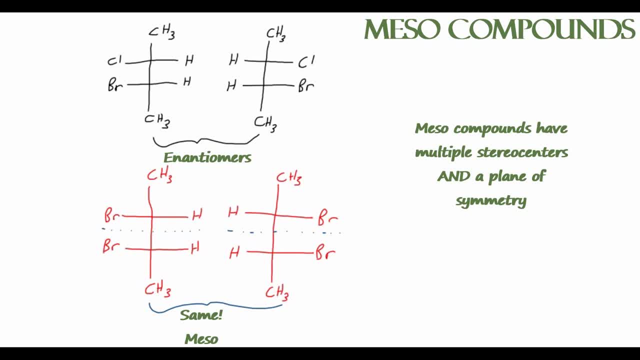 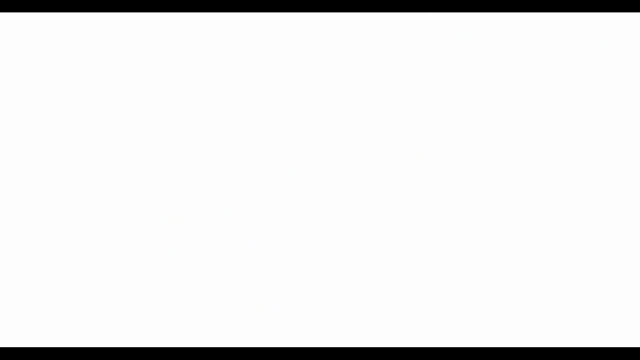 than one stereocenter but that also have a plane of symmetry. So that's important to recognize whenever you have compounds with multiple stereocenters. If I start a new page here, we can also have maybe this substituted cyclobutane, so a cyclic compound of our four-membered ring, And let's draw the two. 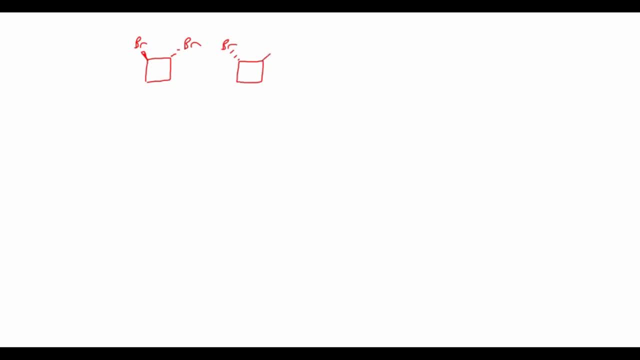 bromine substituents trans to each other, So one will be facing towards us, the other away from us. Again, as with the last one, these two compounds are enantiomers, They are mirror images and they are non-superimposable. 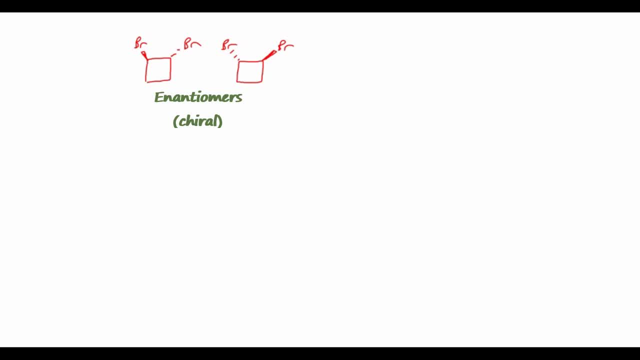 Remember there is no plane of symmetry in this molecule. However, if we draw the same cyclobutane skeleton, except now we have the bromine substituents, cis to each other. So remember cis is the same side And maybe we could consider drawing the mirror image with both of the 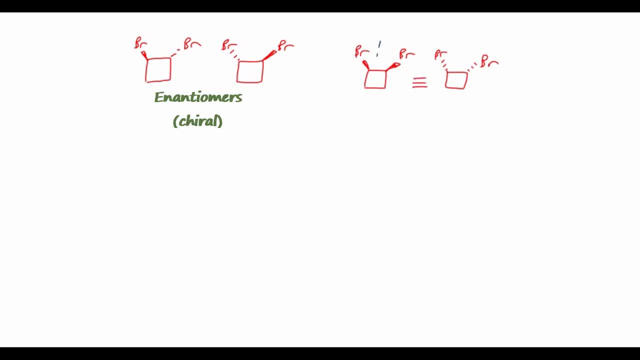 bromines pointing into the page. But if you think about this for a second, these are actually the same molecule again, because you can just flip that molecule over and end up with the first one, So they are superimposable, Which means that again, this second cyclobutane molecule that I've drawn is meso, So it has a plane of. 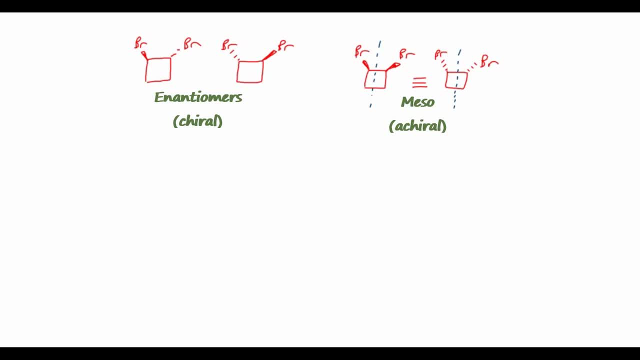 symmetry and it has multiple stereocenters, which means that it does not have an enantiomer. So, to reiterate, if you ever have a molecule with more than one stereocenter, it's always a good idea to look to see if you can find a plane of symmetry. 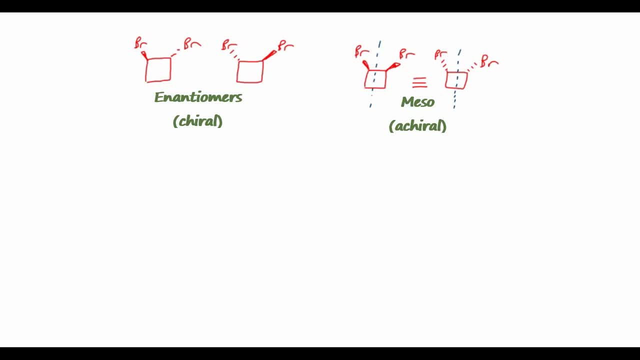 in that molecule, which will signify that it's a meso compound And it actually is achiral, So it's not optically active and it does not possess an enantiomer. So the second topic I'd like to take a look at in this video is chiral resolution or resolution of enantiomers. 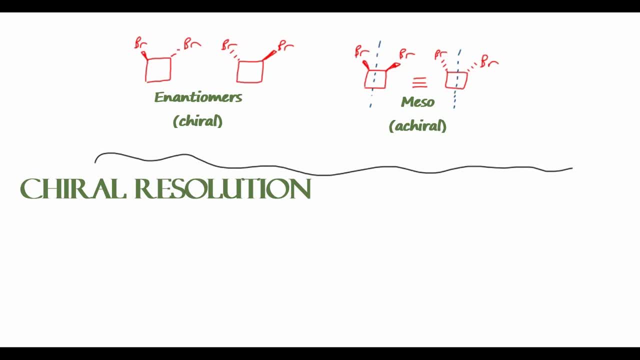 So, basically, these are a set of methods that chemists use to separate a racemic mixture, So racemic being an equal mix of two enantiomers- And all of these methods rely on an enantiomer And they rely on the fact that diastereomers have different physical and chemical properties. 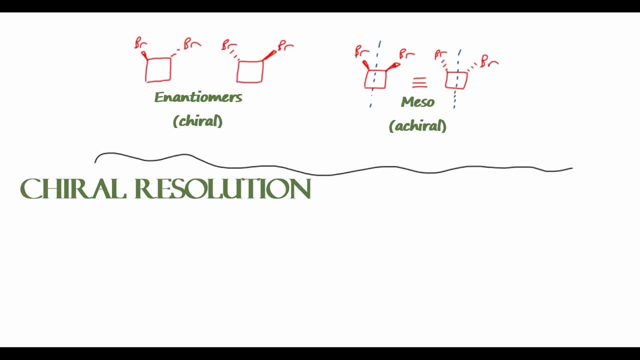 Whereas enantiomers have almost exactly the same physical and chemical properties. So our goal in all of these is to make a diastereomer, separate it and then recover our enantiomers separately. So the first of these methods is called recrystallization. 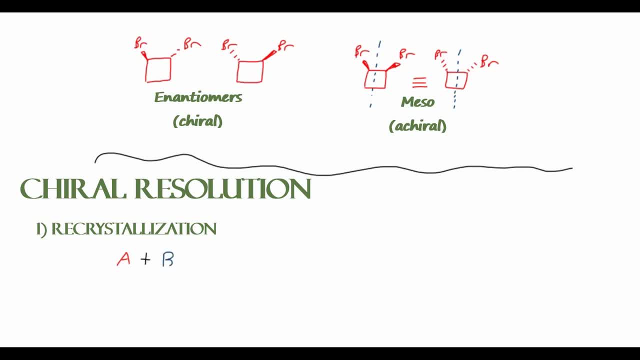 And what recrystallization is is synthesizing a chiral salt. out of First we have a racemic mixture, So let's say A plus B, And an enantiomerically pure compound, C, for example. So we only have one enantiomer of C. 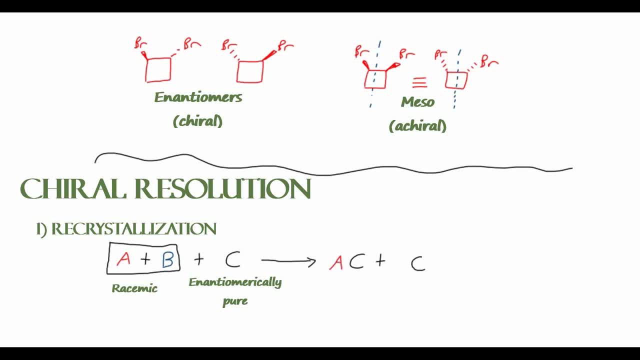 If we form a salt out of those compounds, then what we get is a mixture of diastereomers, Say A, C and B C. Like I said, those diastereomers will have different physical properties, So it's much easier to separate them using conventional means. 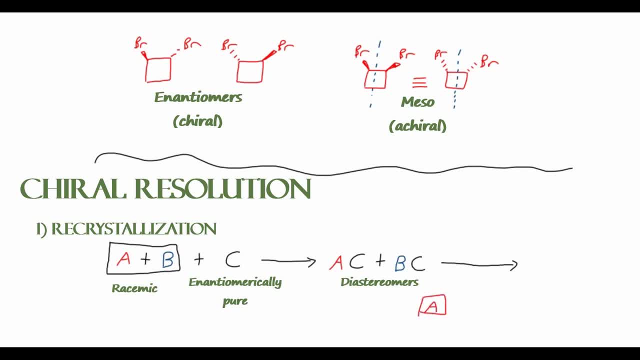 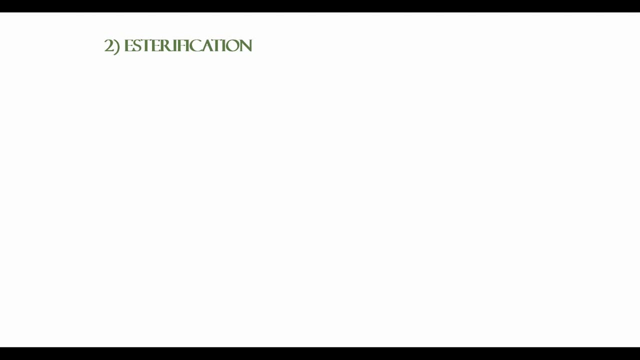 We can separate them and then decompose the salt into its constituents, which will yield us the pure enantiomers A and B separately. Another method is esterification, And this is a reaction that we'll talk about later in the course. 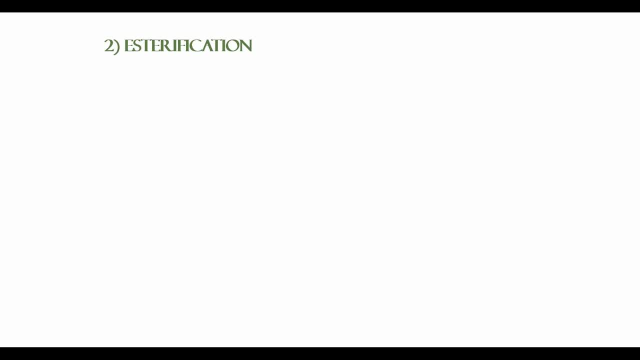 But it involves making an ester, an organic ester, out of a carboxylic acid and an alcohol. So, for example, if we have a racemic mixture of alcohols, let's call them R-A-O-H and R-B-O-H. 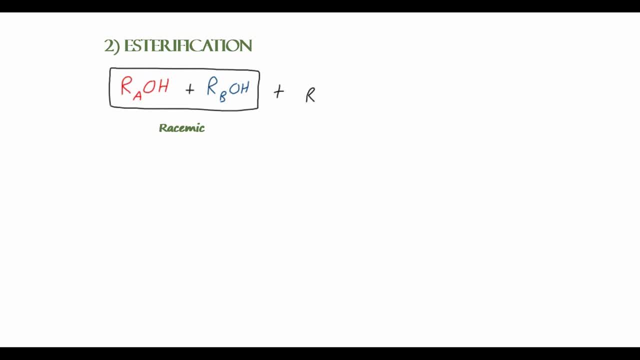 where R is our chiral group and an enantiomerically pure carboxylic acid, we'll call that R prime, with a carboxyl group on the end, And if we convert these into an ester, then again like the last one. 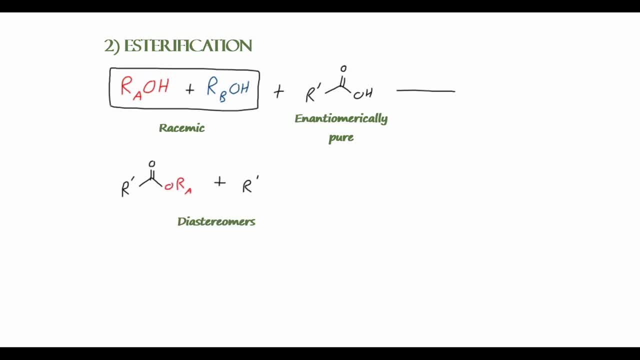 we get a mixture of diastereomers, So a diastereomeric mixture of ester, which we can then separate fairly easily, decompose the ester back into its constituents and recover, now separated, the chiral compounds with the groups R-A and R-B. 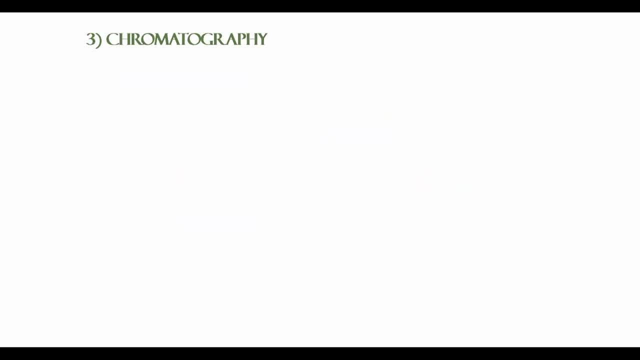 The last method I'll talk about is chromatography. So if you've never had a course on chromatography before or you've never learned anything about it, basically chromatography is a method where we fill a column with what we call a stationary phase. 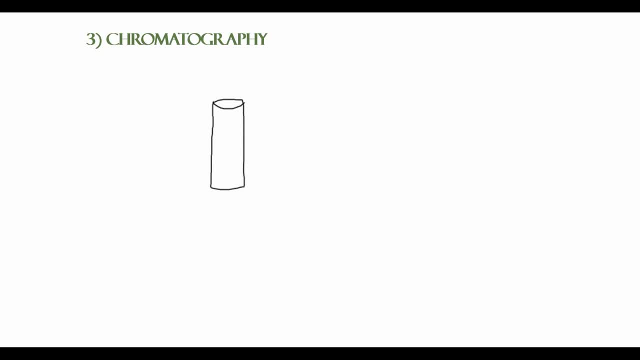 then we insert our sample into the column and, based on the interactions between our sample and whatever is in the stationary phase, different constituents of our sample will come out of the column at different times, So we can separate a mixture of compounds In terms of chiral resolution. 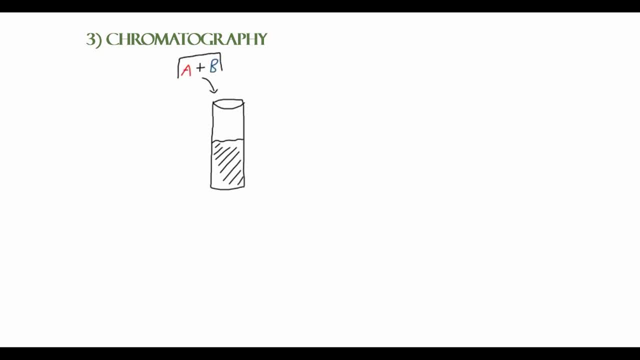 what we can do is have our stationary phase be an enantiomerically pure compound, Just like we've had in the other two methods. Then we insert our sample, so our racemic mixture of A and B, into the column and because our stationary phase is chiral,